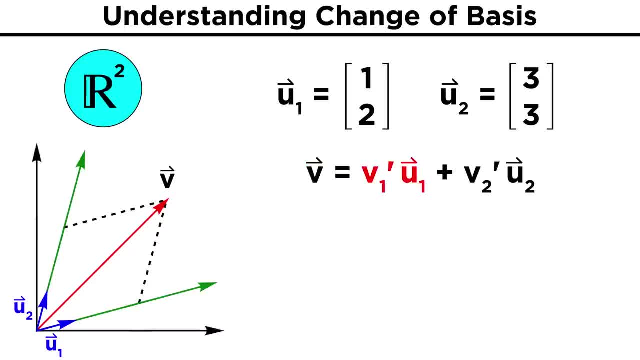 in terms of this basis, where v equals v1 prime u1 plus v2 prime u2, where v1 prime and v2 prime are our new coordinates. in this basis, While we are changing basis, we're not actually affecting the vector, so it is still the same. 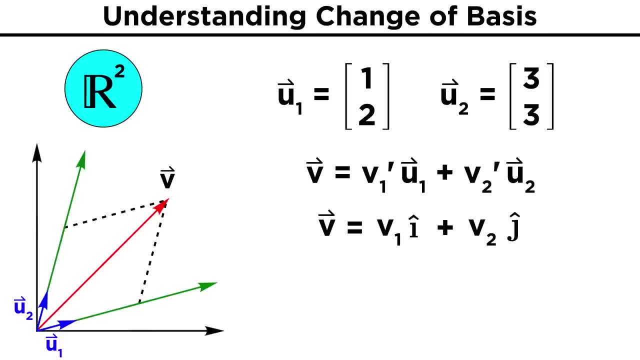 vector as before, when we wrote it as v1 i plus v2 j, meaning we can set these two expressions equal to each other. We can also write our new basis vectors in terms of i and j. u1 equals one zero plus two times zero, one, which is just one i plus two j. 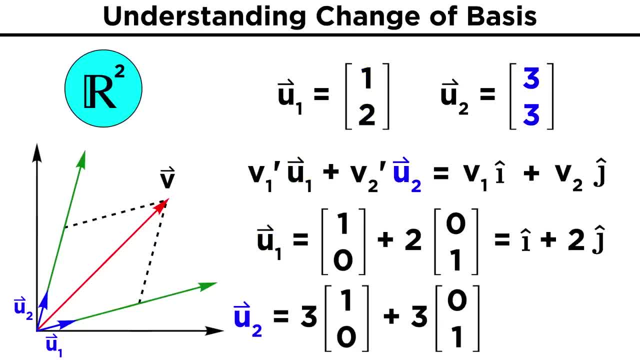 u2 equals three times one zero plus three times zero one, which is just three i plus three j. Now see what happens when we substitute these values into our equation for the vector v. We end up getting v1 i plus v2 j. 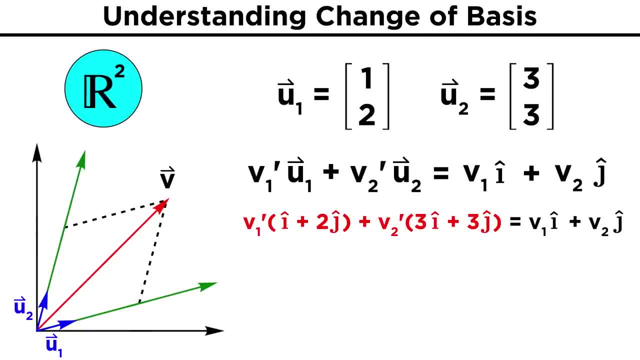 u1 is equal to v1 prime i plus two j plus v2 prime three i plus three j. Doing a little algebra we can quickly distribute these terms and then group in terms of i and j. So this side becomes v1 prime plus three. v2 prime i plus two. v1 prime plus three v2. 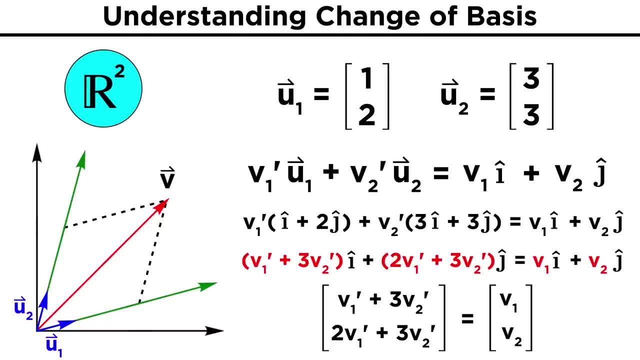 prime j. We can put this back into vector form, since both sides have the same vector form. So we can put this back into vector form, since both sides have the same vector form. since both sides have the same vector form, This raises two questions. 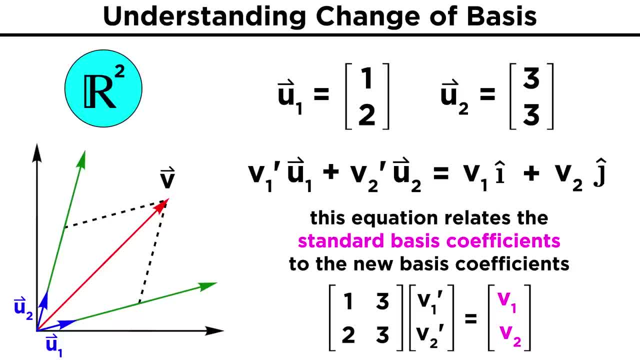 We have two, three c, using the guarantee that v1 is 1 by a度 and v2 is v2 by a度. Both sides have an i-term and a j-term, And then we can write this out as a coefficient matrix multiplied by a vector with components. 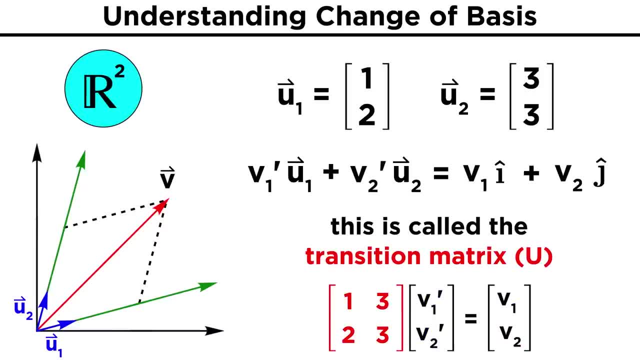 v1 prime and v2 prime. We now have a simple matrix equation that relates the coefficients in our standard basis as the transition matrix represented by the letter U, and we will note that V is equal to U times V prime. An important thing to note is that this transition matrix has columns that are the same as the. 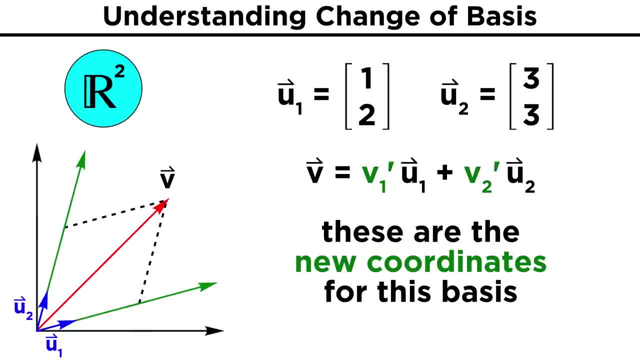 prime u2, where v1- prime and v2- prime are our new coordinates in this basis. While we are changing basis, we're not actually affecting the vector, so it is still the same vector as before, when we wrote it as v1i plus v2j, meaning we can set these two expressions. 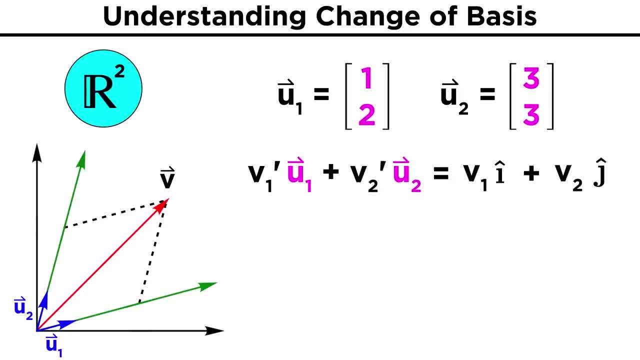 equal to each other. We can also write our new basis vectors in terms of i and j: u1 equals, which is just, u2 equals plus, which is just Now. see what happens when we substitute these values into our equation for the vector v. 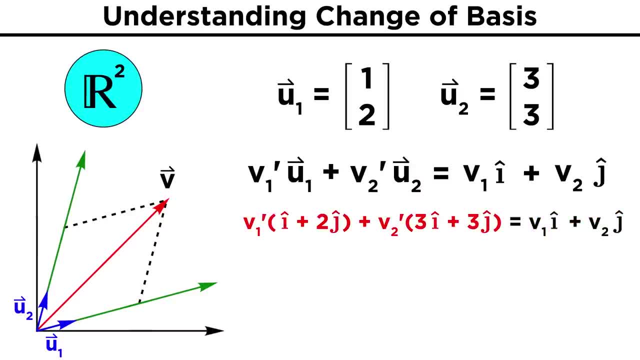 We end up getting v1i plus v2j. We can also write our new basis vectors in terms of i and j, U1 equals plus plus v2j, being equal to v1 prime i plus 2j plus v2 prime 3i plus 3j. 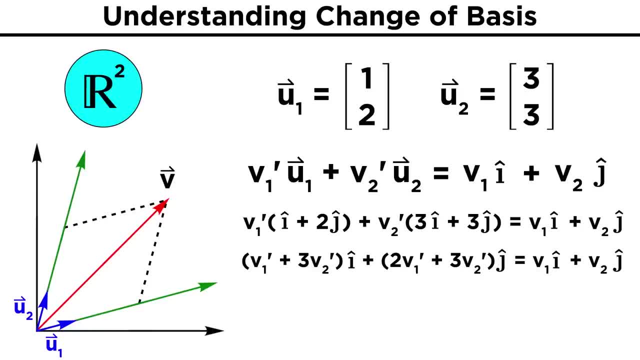 Doing a little algebra we can quickly distribute these terms and then group in terms of i and j. So this side becomes v1 prime plus 3v2 prime i plus 2v1 prime plus 3v2 prime j. 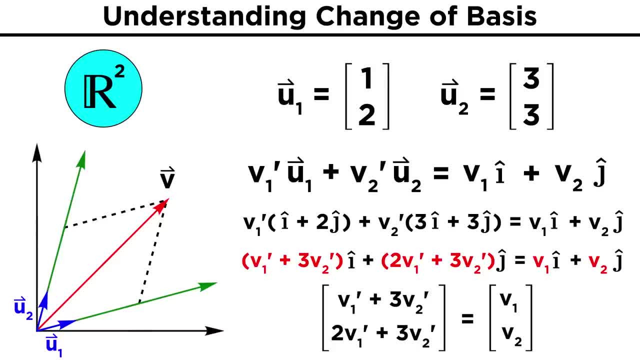 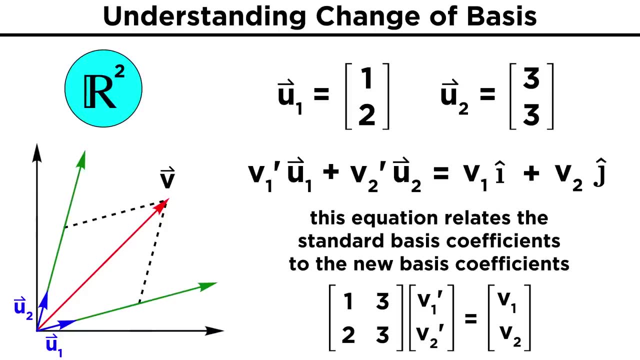 We can put this back into vector form, since both sides have an i term and a j term, And then we can write this out as a coefficient matrix multiplied by a vector with components v1 prime and v2 prime. We now have a simple matrix equation that relates the coefficients in our standard basis. 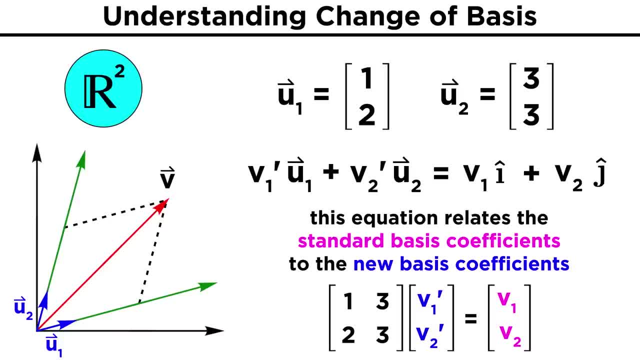 v1 and v2, to the coefficients in our new basis, v1 prime and v2 prime. The matrix that relates them is referred to as the transition matrix, represented by the letter u, and we will note that v is equal to u times v prime. 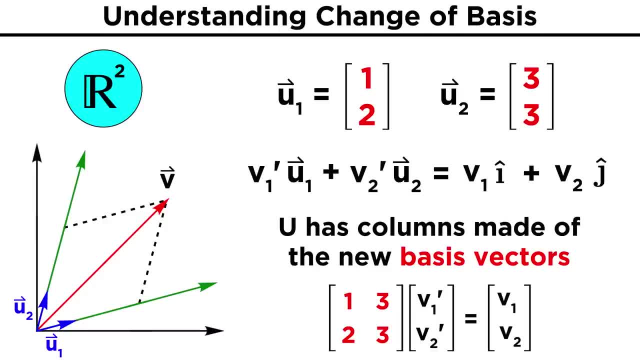 An important thing to note is that this transition matrix has columns that are the same as the basis, vectors u1 and u2.. This means that, in order to easily get the transition matrix between any basis and the standard basis, instead of going through the algebra each time, the matrix u can be written as the new. 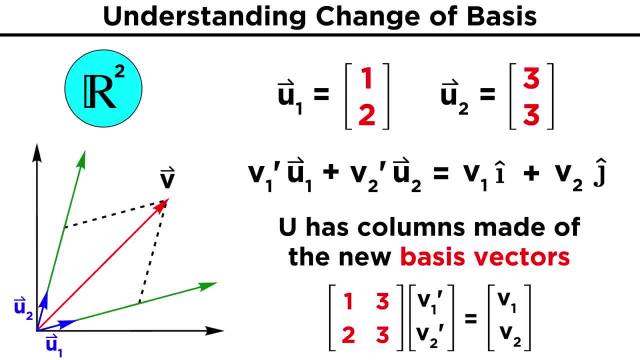 basis, vectors U1 and U2.. This means that, in order to easily get the transition matrix between any basis and the standard basis, instead of going through the algebra each time, the matrix U can be written as the new basis we are working with as its columns. 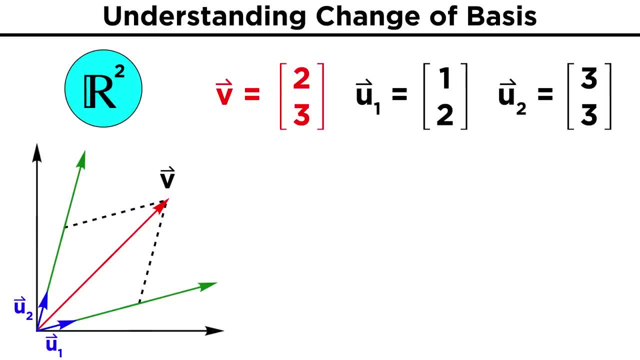 Finally, let's say we started with a vector. in the standard basis V equals two, three. We want to find the new coefficients in the basis U1, U2.. In other words, we want to solve for V1 prime and V2 prime. 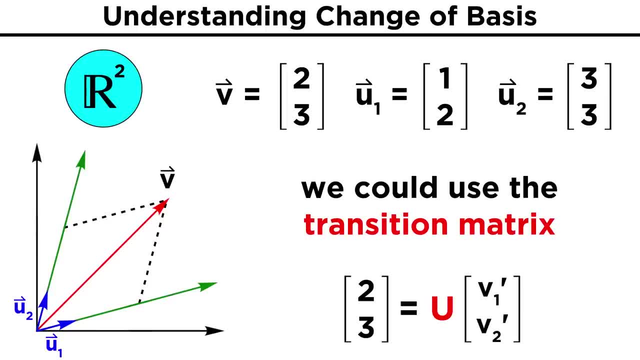 We could jump straight to using the transition matrix. But to make things even easier, we can manipulate this equation such that V1 prime and V2 prime are isolated. In order to isolate this V prime term, we have to get rid of U. Remember that when we 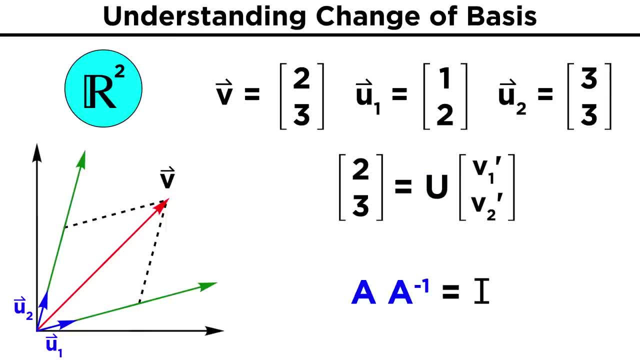 learned about inverse matrices. a matrix multiplied by its inverse will give the identity matrix, or effectively just the number one, Just like dividing some number by itself. Let's therefore multiply our equation by the inverse. Let's therefore multiply our equation by the inverse. 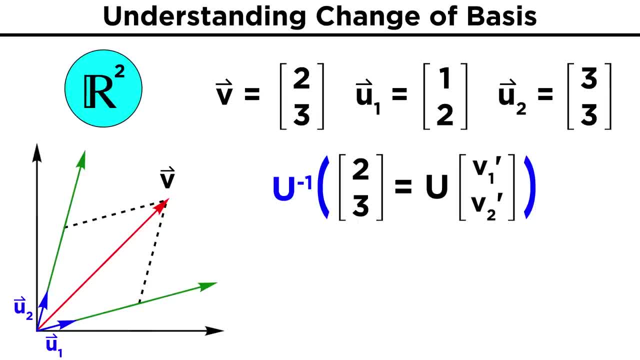 Let's therefore multiply our equation by the inverse of U, which is labeled U, to the negative one. Bear in mind that order matters in matrix multiplication. it is not commutative, So let's make sure to make U inverse the leftmost term on each side of the equation. 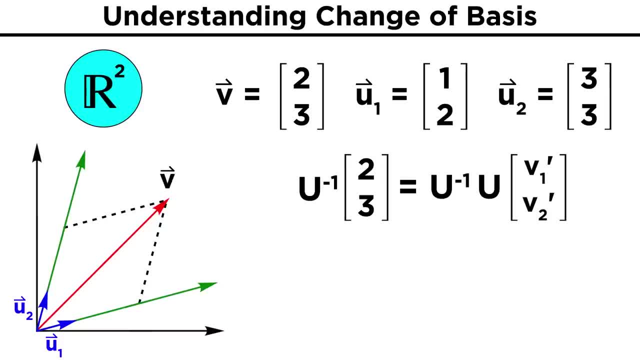 We end up with U inverse, V equals U inverse, U V prime And since U inverse and U multiply to become one, we get one V prime or simply V prime on the right side. Now we can plug in our numbers. We know our transition matrix is one, three, two, three and the vector we want to change. 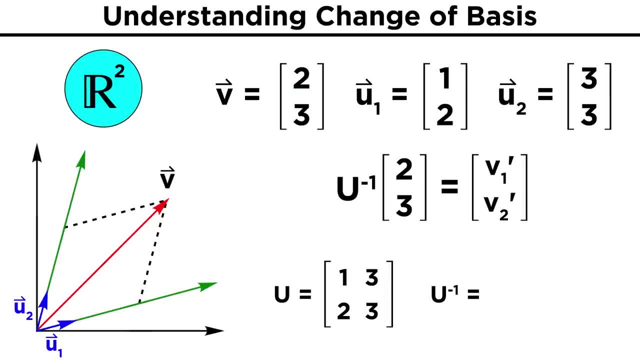 basis for is two, three. We will need the inverse of the transition matrix, since the equation calls for U inverse times V. so for a two by two matrix, we simply switch the diagonal terms, flip the sign on the other terms and then divide this by the determinant of the original matrix. 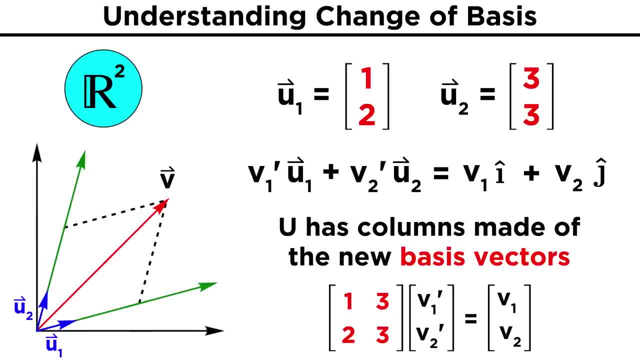 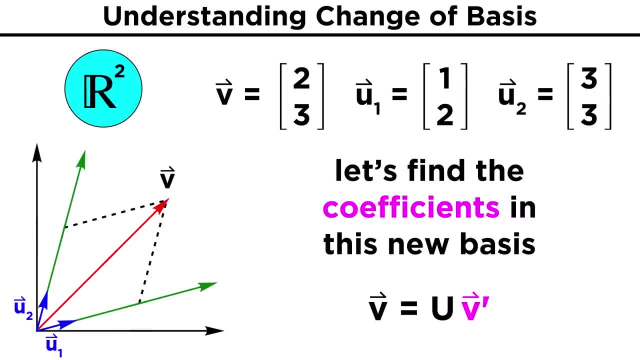 basis we are working with as its columns. Finally, let's say we started with a vector. in the standard basis, v equals two, three. We want to find the new coefficients in the basis u1, u2.. In other words, we want to solve for v1 prime and v2 prime. 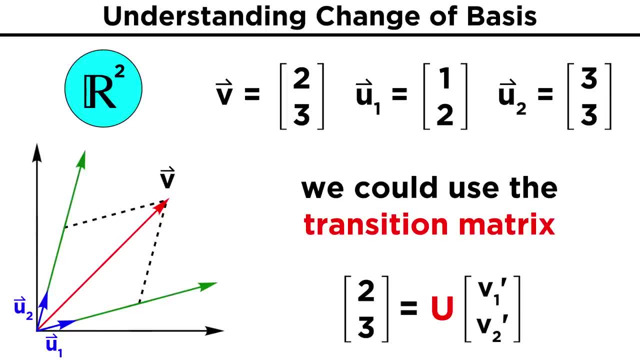 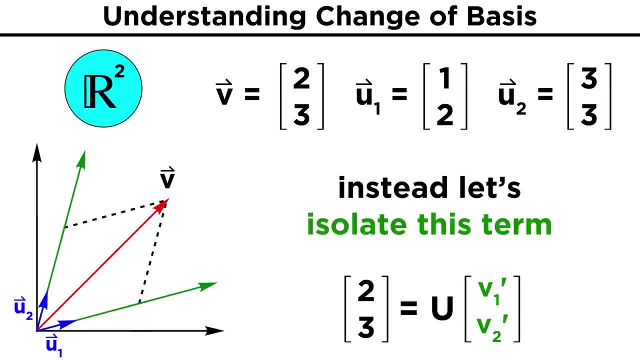 we could use the transition matrix. but to make things even easier, we can manipulate this equation such that v1 prime and v2 prime are isolated. In order to isolate this v prime term, we have to get rid of? u Remember that when we learned about inverse matrices, a matrix multiplied by its inverse 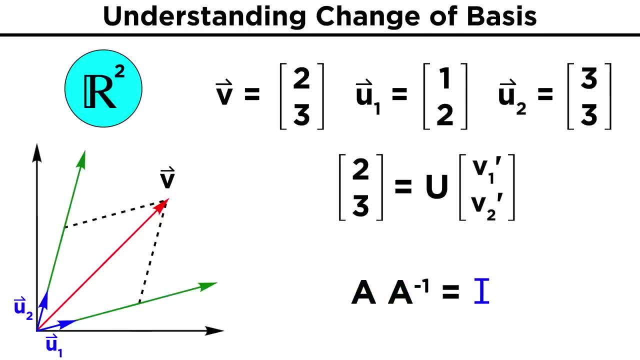 will give the identity matrix, or effectively just the number one, just like dividing some number by itself. Let's therefore multiply our equation by the inverse of u, which is equal to u, times u, Which is labeled u, to the negative one. Bear in mind that order matters in matrix multiplication. it is not commutative. 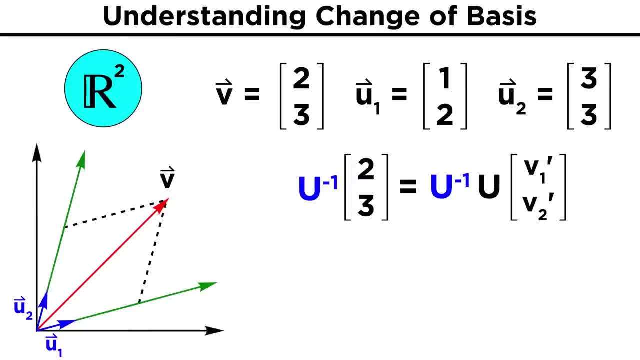 So let's make sure to make u inverse the leftmost term on each side of the equation. We end up with u inverse, v equals, u inverse, u v prime, And since u inverse and u multiply to become one, we get one v prime, or simply v prime. 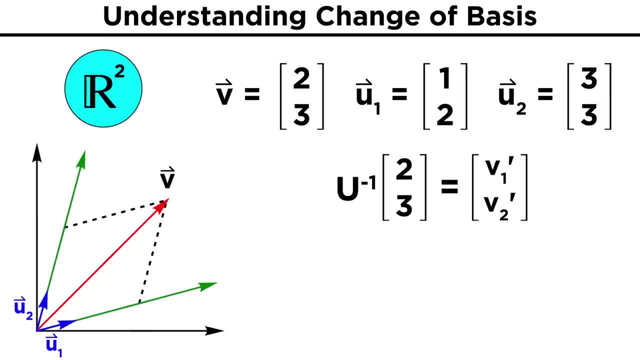 on the right side. Now we can plug in our numbers. We know our transition matrix is one, three, two, three And the vector we want to change basis for is two, three. We will need the inverse of the transition matrix, since the equation calls for u inverse. 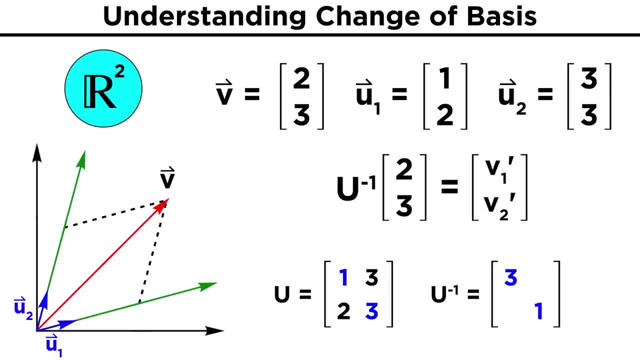 times v. so for a two by two matrix, we simply switch the diagonal terms, flip the sign on the other terms and then divide this by the determinant of the original matrix. We find that the determinant of u is negative three and this will give us an inverse matrix. 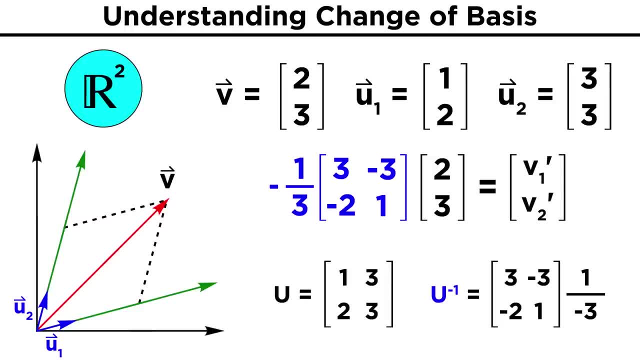 of three negative, three negative two, one, all multiplied by negative one third. Now let's plug in our vector v, which was two, three. Going through the matrix multiplication, we get these expressions which we can simplify, and then each term will be multiplied by negative one third. 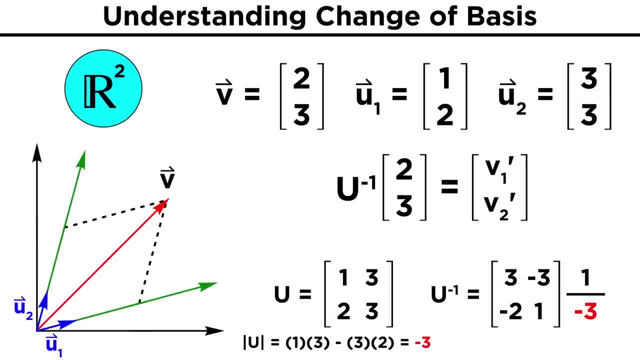 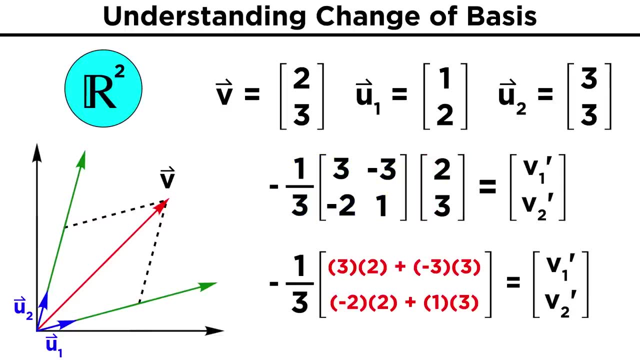 We find that the determinant of U is negative three, and this will give us an inverse matrix of three negative three, negative two, one, all multiplied by negative one, third. Now let's plug in our vector V, which was two, three. 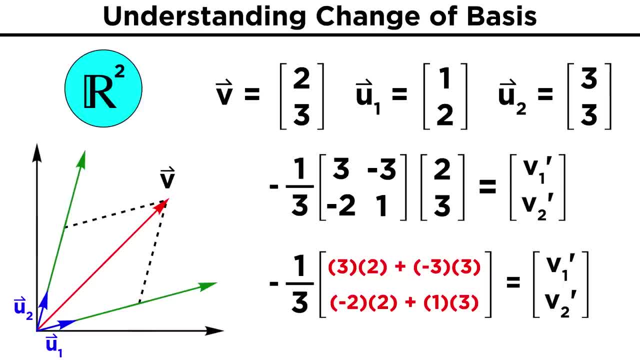 Going through the matrix multiplication, we get these expressions which we can simplify, and then each term will be multiplied by negative one third. This leaves us with V prime equals U. V prime equals one one third. These are the new coordinates of V in the basis: U one, U two. 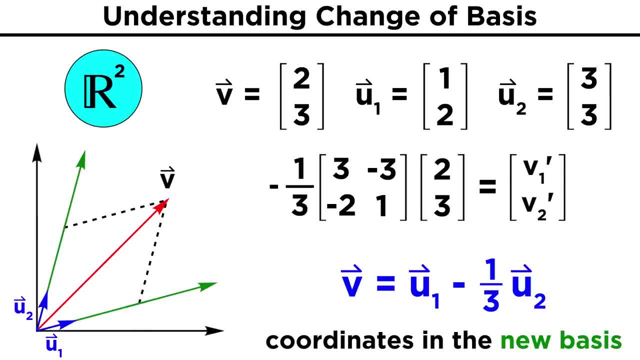 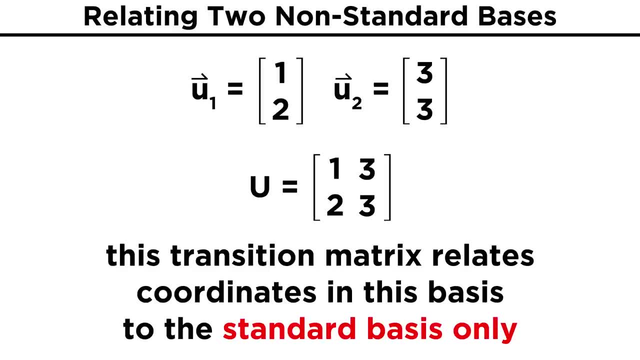 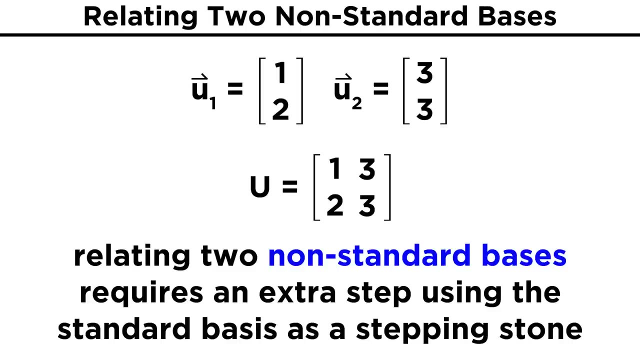 Written out this is: V equals U one minus one third U two. It's important to note that the transition matrix made of the basis vectors as columns relates the coordinates in that basis to the standard basis only Relating to non-standard bases. Relating to non-standard bases requires an extra step, using the standard basis as a stepping. 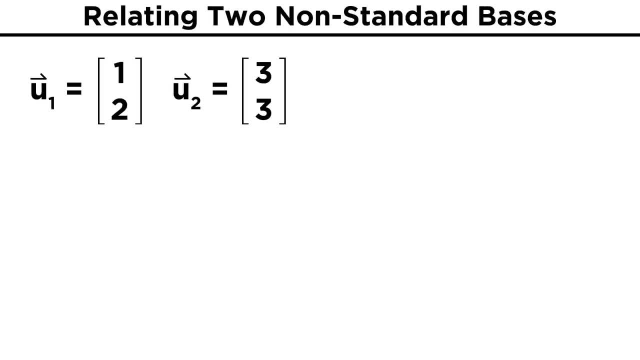 stone. Let's say, in addition to our basis, U one equals one, two and U two equals three, three- we also have a basis W one equals negative one, negative one, and W two equals three zero. We know that the transition matrix for each basis- U and W- will relate each to the standard. 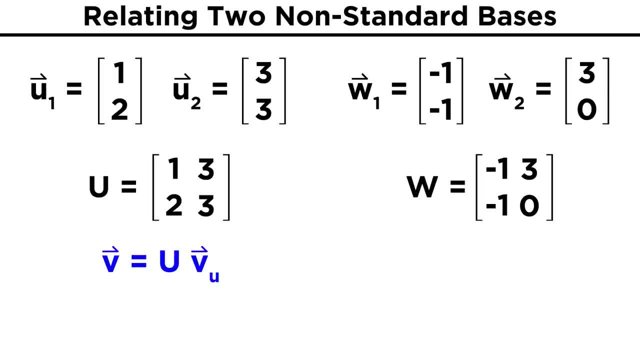 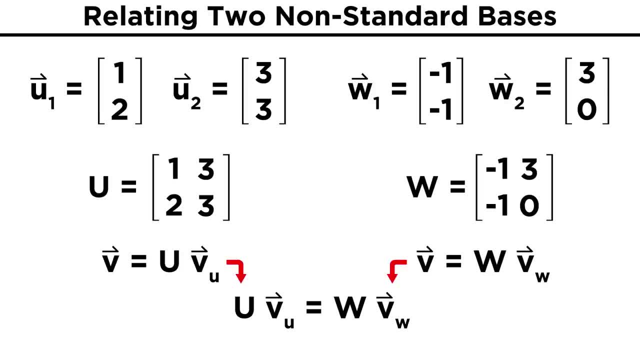 Setting these two equal to one another. we get U V U equals W V W, which makes getting from one basis to another as easy as taking an inverse matrix Going from W to U. we get V? U equals U. inverse W V W. 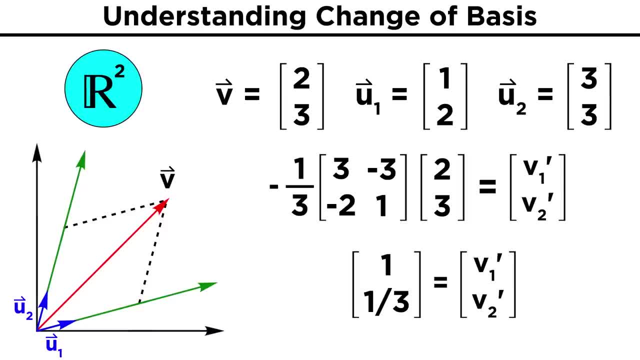 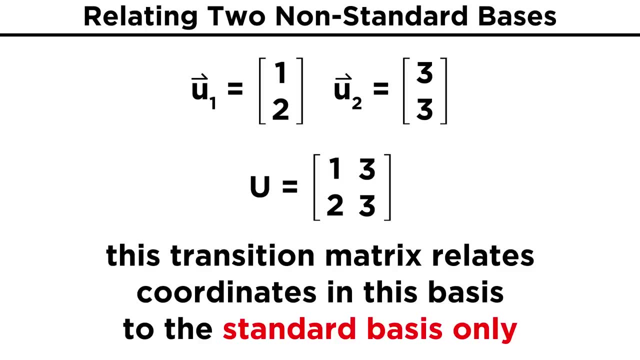 This leaves us with v prime equals one-third. These are the new coordinates of v in the basis: u one, u two. Written out, this is: v equals u one minus one-third u two. It's important to note that the transition matrix made of the basis vectors as columns. 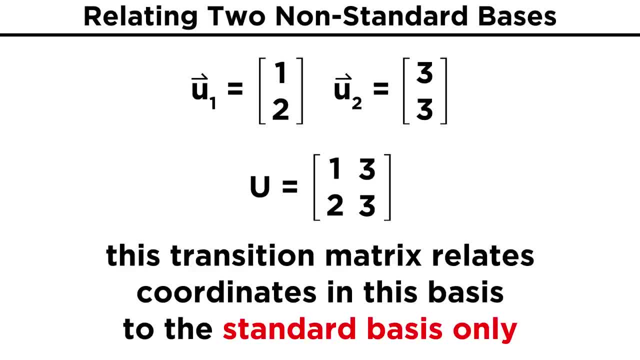 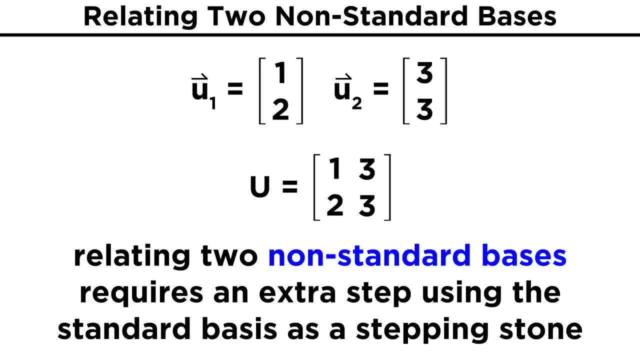 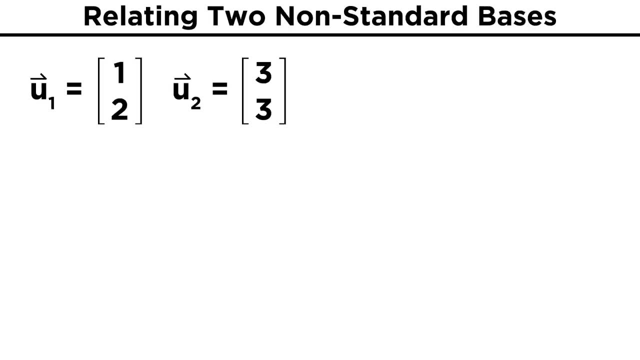 relates the coordinates in that basis to the standard basis only. Relating two non-standard bases requires a new matrix. It requires an extra step, using the standard basis as a stepping stone. Let's say, in addition to our basis, u one equals one, two and u two equals three, three. 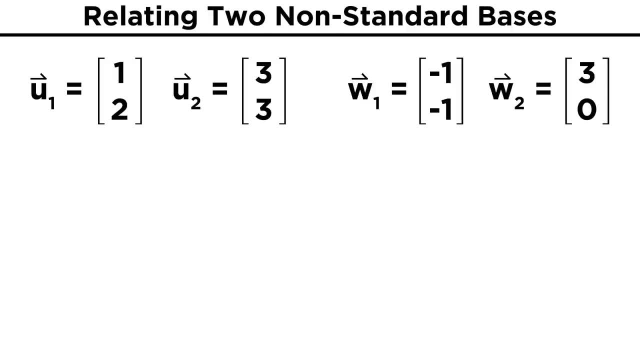 we also have a basis: w one equals negative, one negative one and w two equals three zero. We know that the transition matrix for each basis- u and w- will relate each to the standard basis, Relating the standard basis to the u basis. we know that the transition matrix for each 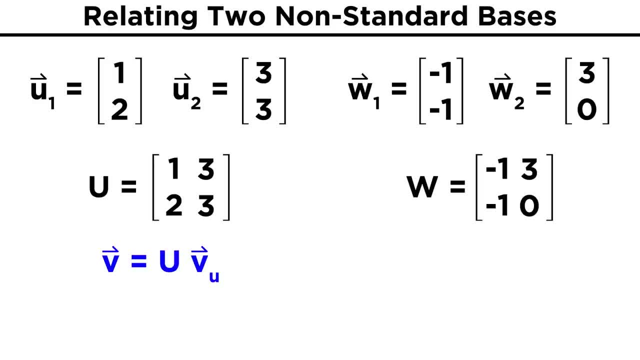 basis u and w will relate each to the standard basis. We know that the transition matrix for each basis v equals u v u And relating the standard basis to the w basis, v equals w v w. Setting these two equal to one another, we get u v u equals w v w, which makes getting 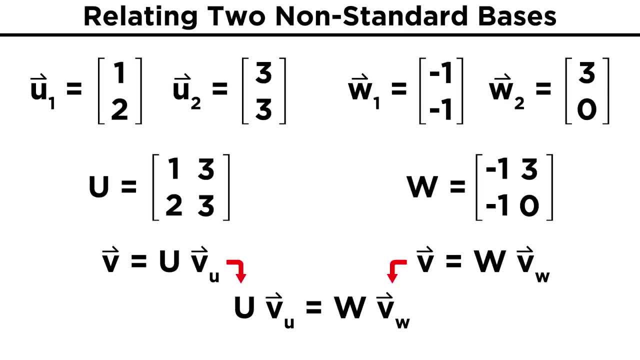 from one basis to another. as easy as taking an inverse matrix. Going from w to u, we get v? u equals u- inverse w v w. From w to w, we get v? w equals w inverse u v u. This change of basis is actually a kind of linear transformation which we will be covering. 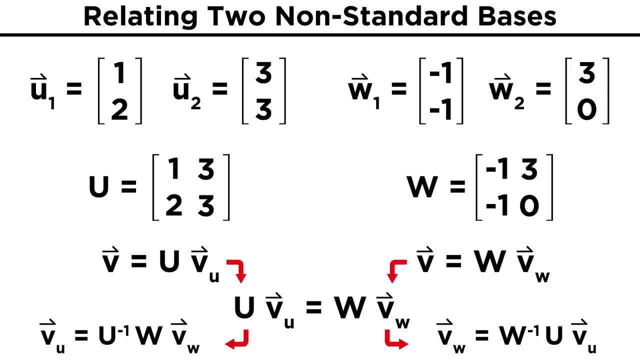 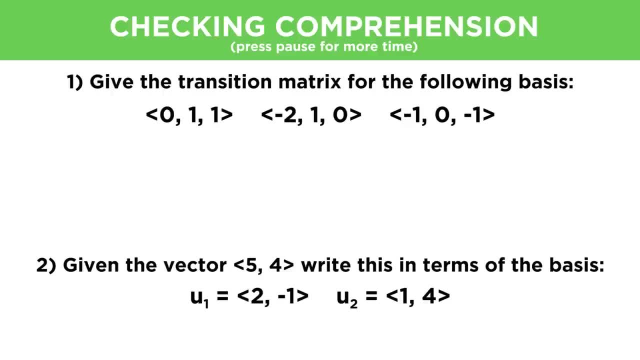 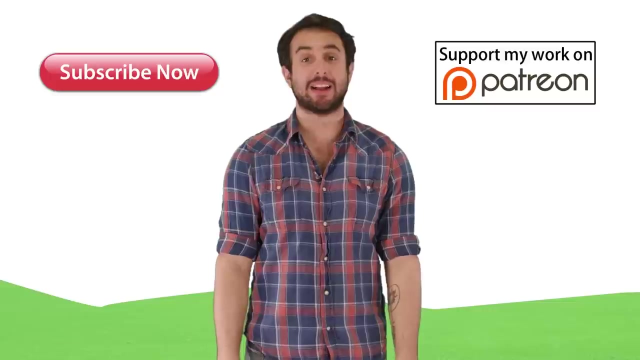 next, but before moving on, let's check comprehension. Thanks for watching, guys. subscribe to my channel for more tutorials. support me on patreon so I can keep making content and, as always, feel free to email me. professordaveexplains.